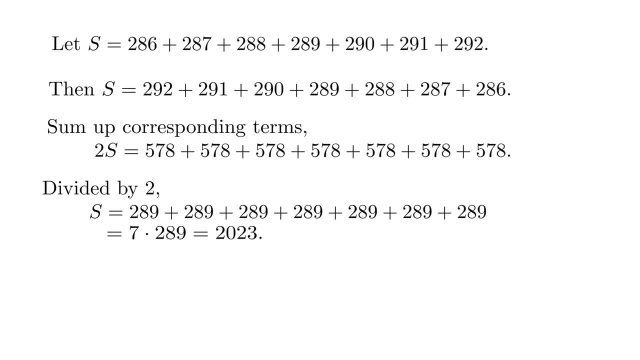 In this case, 7 is a factor of 2023.. Secondly, we can calculate the sum of a sequence of consecutive integers by sum up the first term and the last term and multiply the number of terms divided by 2.. This formula is also applicable to every arithmetic sequence. 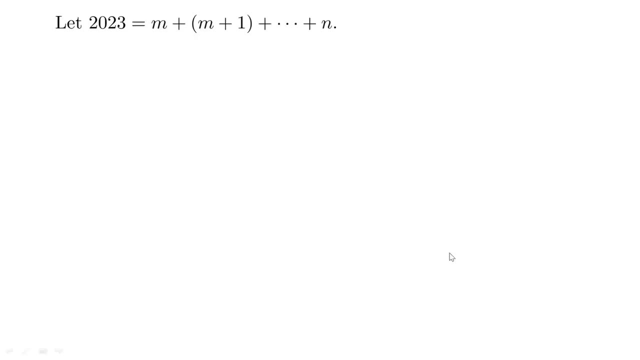 Let 2023 be the sum of integers. Let 2023 be the sum of integers from m to n, Then 2023 equals the first number plus the last number, that is, m plus n, multiplied by the number of terms, n minus m plus 1, divided by 2.. 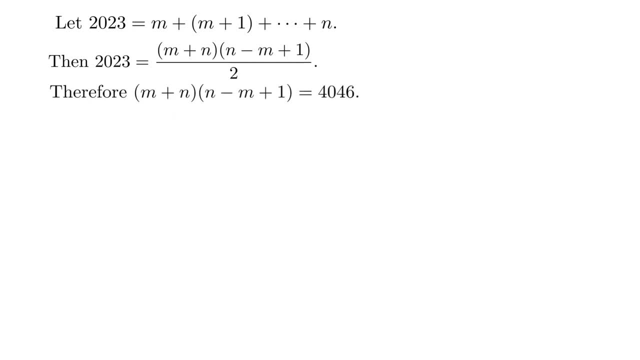 Therefore, m plus n times n minus m plus 1 equals 4046.. Well, m can be negative, m plus n must be positive, And the number of terms n minus m plus 1 is also positive. Therefore, both m plus n and n minus m plus 1 are positive factors of 4046. 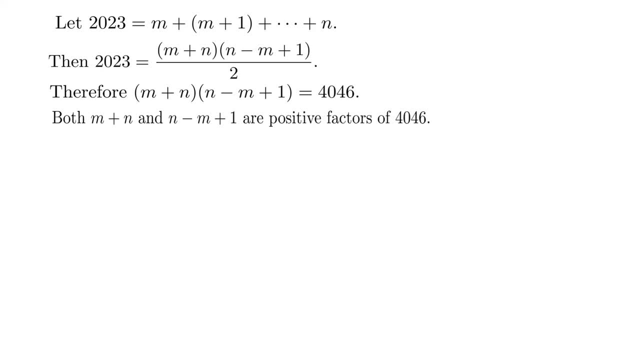 Let's list all of the factors of 4046.. This is related to prime factorization of 4046, which is 2 times 7 times 17 squared. The factors of 4046 are different choices of these prime factors. There are a total of 12 combinations. 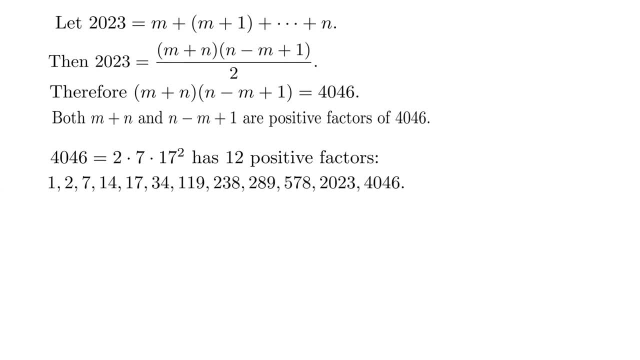 These are the factors, from 1 to 7 all the way to 4046.. Total of 12 of them. The number of terms n minus m plus 1 must be one of the factors. There are a total of 12 cases. 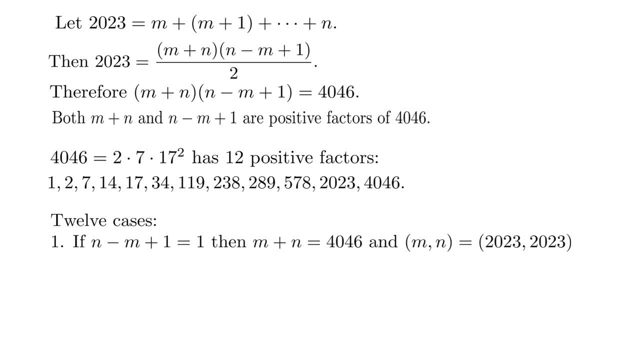 The first case: there's only one term: n minus m plus 1 equals 1.. Only one term. This term must be 2023.. Second case: if there are two terms, then m plus n equals 2023.. Only two numbers, and one of them is 1011.. 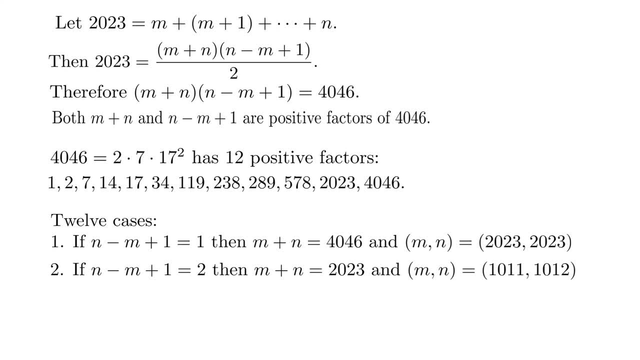 The other is 1012.. The next case: there are seven terms: n minus m plus 1 equals 7, and m plus n equals 578.. The multiplication of these two numbers is 2023.. So this is actually a system of equations in m and n. 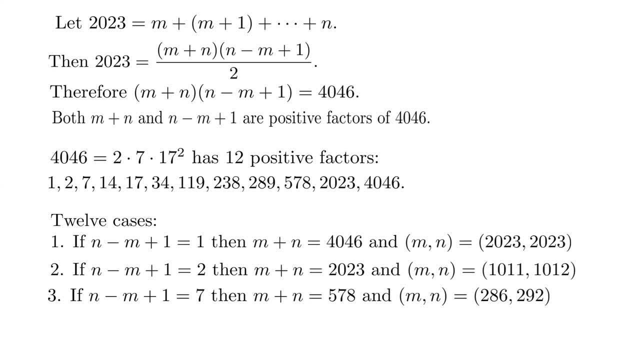 We solve for them: m is 286, n equals 292.. We see this example before We can solve all these equations. The last one would be the number of terms equals 4046.. So, starting from negative 2022 to all the way to positive 2023. 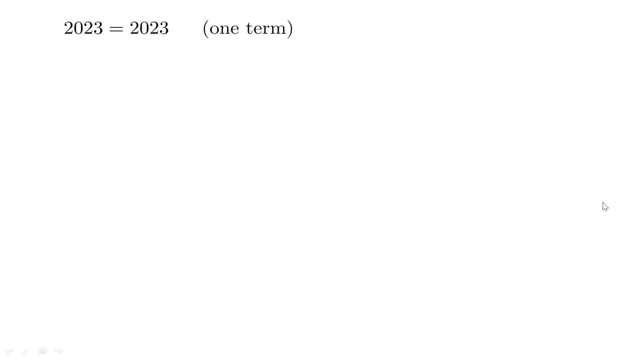 Let's look at all the solutions. The first one: there's only one term, Of course, that is 2023.. If there are two terms, we've seen this before: 1011 plus 1012.. And next one: seven terms. 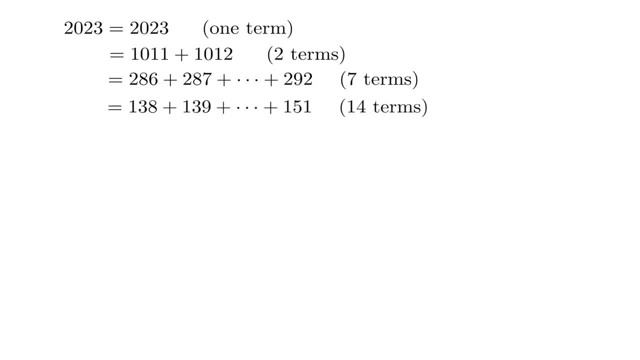 And it can also be 14 terms, starting from 138 to 151.. And the next one, there are 17 terms, from 111 to 127.. And the next one We have 34 terms from 43 to 76.. So far we have six solutions.